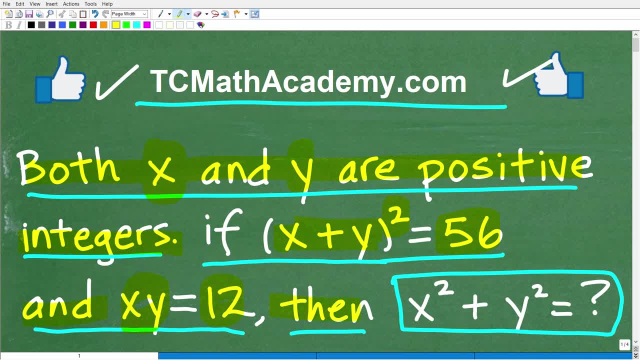 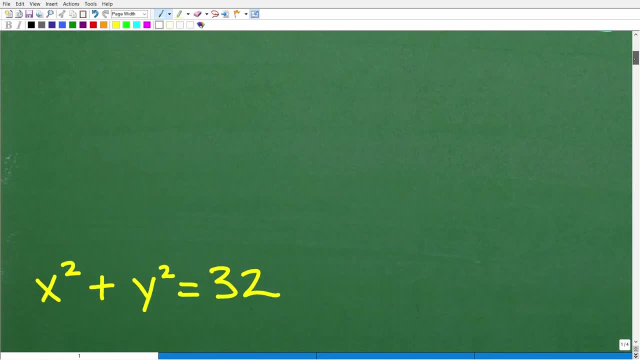 and X times Y is equal to 12, then what is X squared plus Y squared equal to? All right, So that is the question. Let's go ahead and take a look at the answer. X squared plus Y squared is equal to 32.. All right, Well, if you got this right. 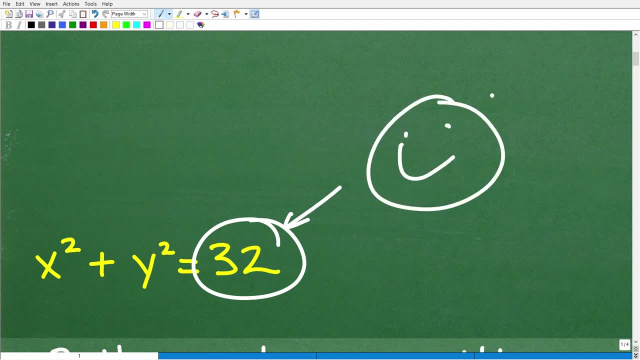 okay, that is very impressive. Matter of fact, I'm going to give you a nice little happy face: an A plus plus 200%. Matter of fact, if you were in my math class or like an algebra class that I was teaching, I would say: take the rest of the year off. I don't know how. 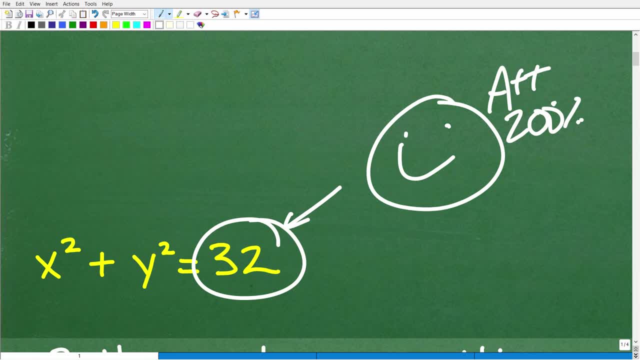 you're getting so good at math- Maybe you're watching that guy on YouTube, But in all, I'm going to give you a nice little happy face and A plus plus 200%. In all seriousness, if you figured this out, that is very good, And there's different approaches. 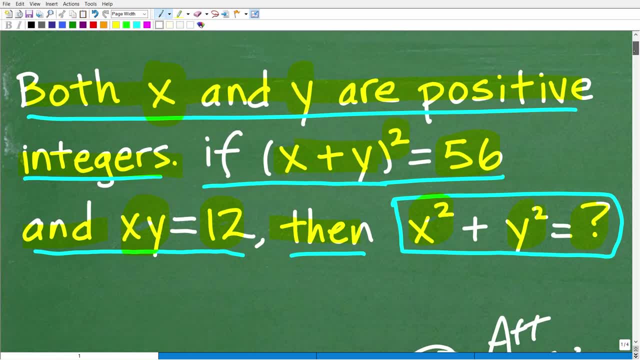 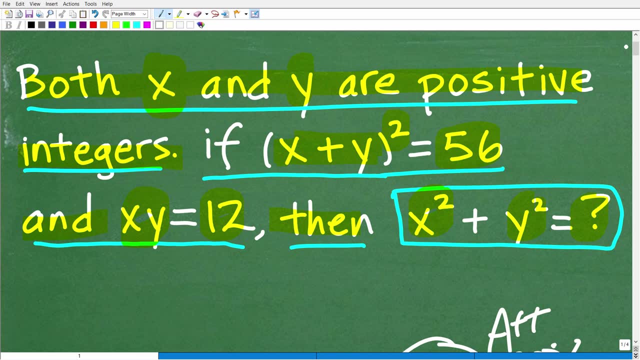 you could take to figure this problem out. Of course, I said that. what I think makes this problem particularly interesting is that the easiest way, in my opinion, is not going to be the most obvious way, But let's go ahead and get into the solution right now. Okay, So we are. 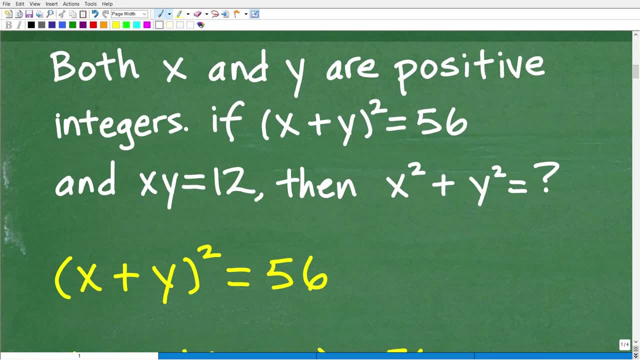 dealing with a math word problem that has a lot of information. So make sure you read this thing at least a few times. And if you're looking at the problem, the problem is stating what is x squared plus y squared equal to right. So this is. 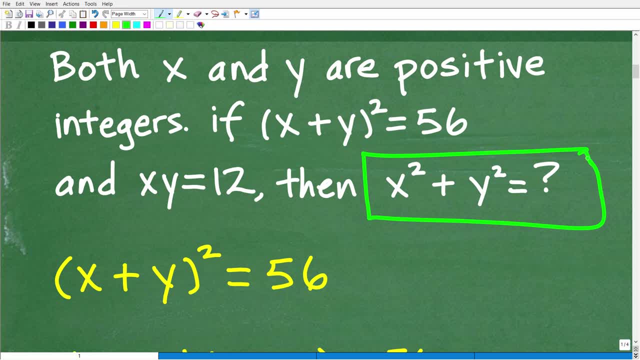 the question in the problem. So we're saying: well, x squared plus y squared is equal to what value? Well, it's probably a good idea for us to start thinking: well, maybe we need to solve for the actual values for x and y, right? So we're like, well, okay, well, I have to figure out what. 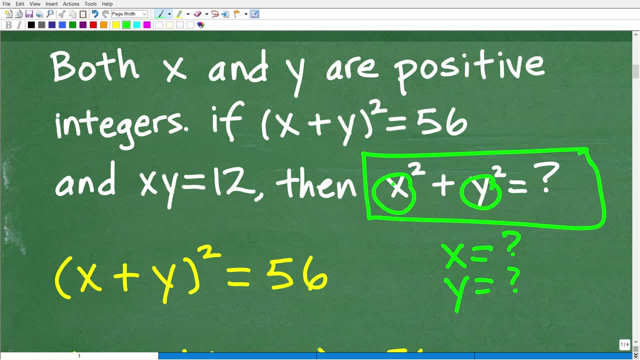 x is equal to and y is equal to. So if I have these values, I could just kind of plug them in and square them and then, you know, solve the problem right. So that is, you know, a logical, common sense type of approach. So if you're thinking in those, 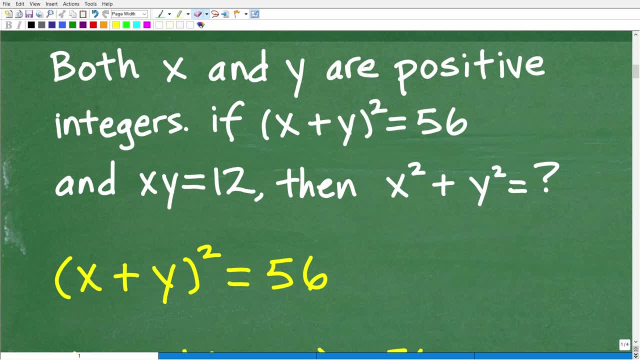 terms. those are good terms, And you might be saying, all right, well, if I got to solve for both x and y, what do I have here that can help me do this? Well, what we have is two equations. So we have x plus y, squared is equal to 56. And we have x, y is equal to 12.. So maybe we could. 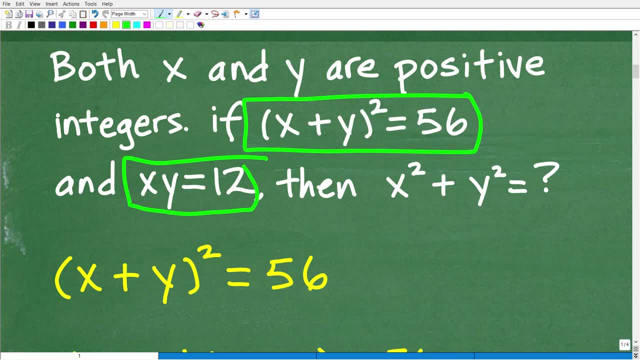 set up a system of equation or use some sort of algebra substitution to solve for x and y, And you could do that. okay, You certainly could do that, But I think this is not the easiest approach. okay, I mean, this is one approach, And if you took that approach, 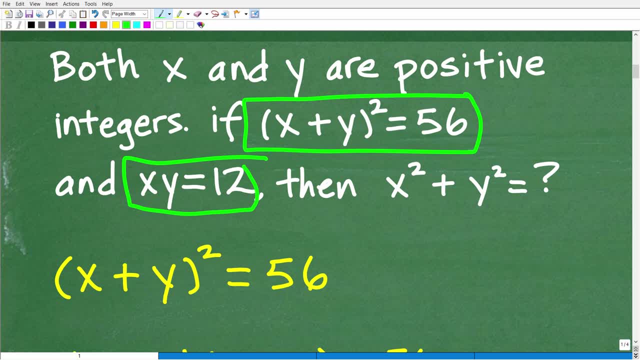 that is fantastic, But sometimes problems like this are designed for you to look for patterns to make your life easy. okay, Or at least easier. A problem like this, by the way, would be something pretty typical of a standardized test like a college entrance exam, like the. 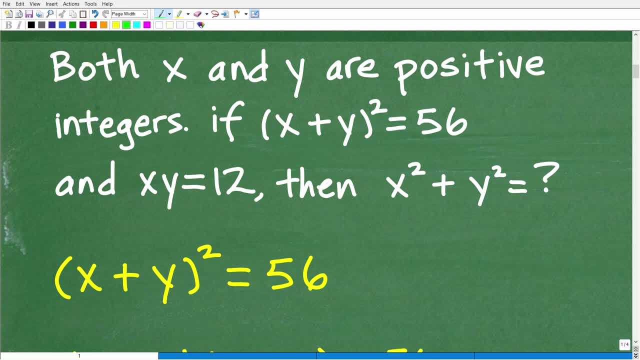 SAT or ACT test. These are a very common type of questions And you'll see why here in a second. because they want you to take a different approach. that's not the most direct approach. okay, In other words, again, most people or students might be saying, okay, I got to solve. 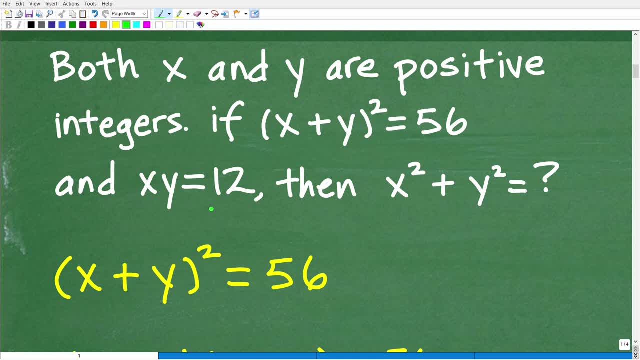 for x and y. So let me go ahead and just start the problem and start plugging in or using the substitution method and start doing a lot of algebra to figure this out. But maybe there is a quicker, faster way, And actually there is. So what we're going to do is we're going to do a 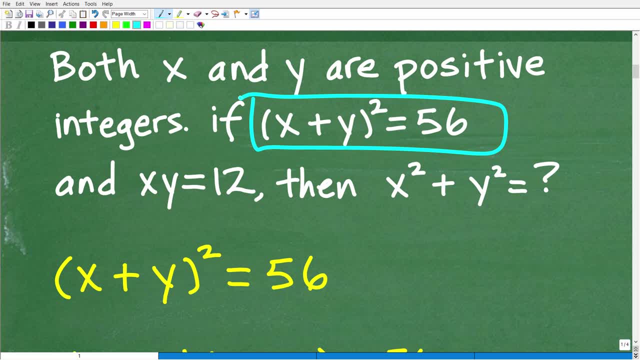 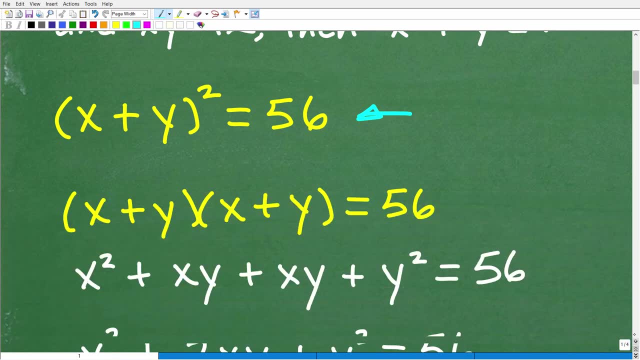 take this part of the problem right here: x plus y squared is equal to 56.. And we're going to, just for a quick second, say you know what? let me do some algebra real quick. I want to take this: x plus. 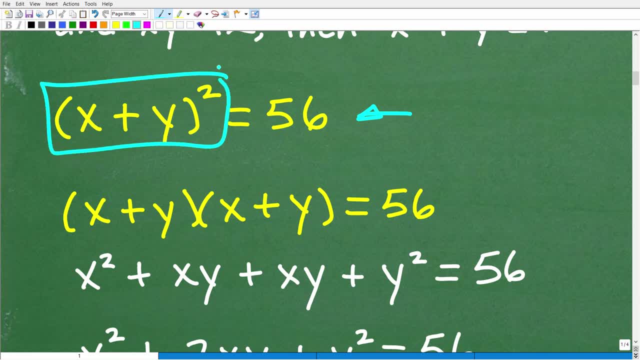 y squared, and I'm actually going to expand that. So what does x plus y squared mean? Well, it means take x plus y and multiply it by itself. So x plus y squared means take x plus y and multiply it by x plus y. So hopefully you remember a bit of algebra. 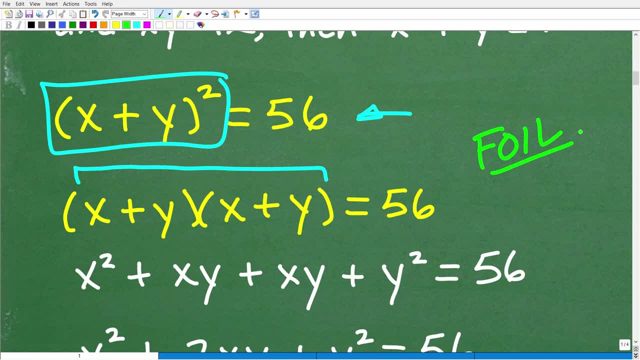 Let's do something called the FOIL method, which is a technique to multiply two binomials. This is what this is. This is a binomial, It's a two-term polynomial, But hopefully you know how to multiply x plus y times, x plus y. Now the FOIL method. this is just an acronym. It stands for first: 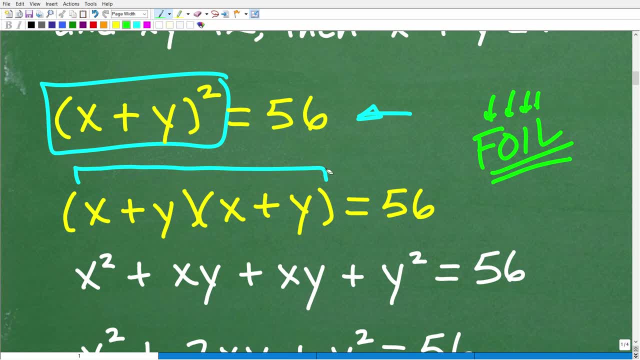 outer inner last, And let me go ahead and explain this to you right now. Okay, so first means multiply the first terms, That's x times x, right? These are the first terms of these binomials. x times x is x squared. The O means multiply the outer terms, So the outer terms is x and y. 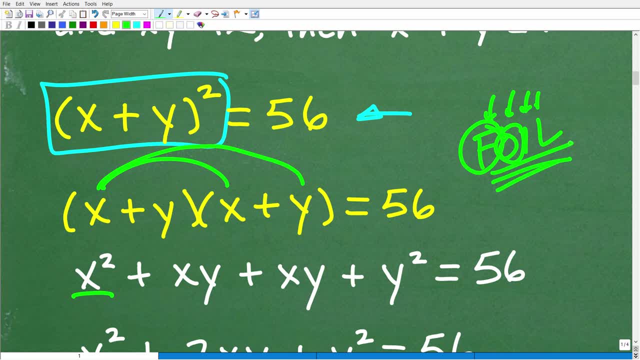 okay, of these two binomials I'm just doing a quick review. If you need more help with this algebra, I'll give you some recommendations once we finish up this video. But x times y is the outer, So that's xy. So i is the inner, So that's y times x. So y times x is the same thing as x. 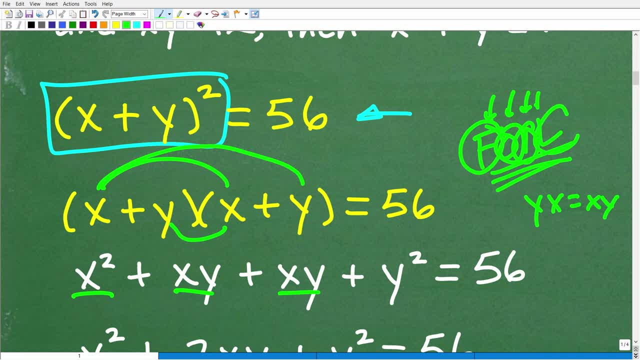 times y. So I'm going to write that as xy, And then l is the lower term, So that's y times x. So the last terms here is y and y. So that would be y times y, which is y squared. Okay, so what? 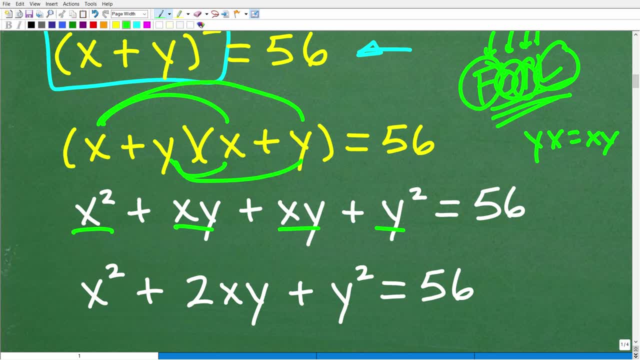 do we have here? Well, we have x squared plus 1xy, plus another 1xy plus y squared, So I can combine these like terms. So if I have a 1xy here and 1xy here, I have a total of 2xy. So we have 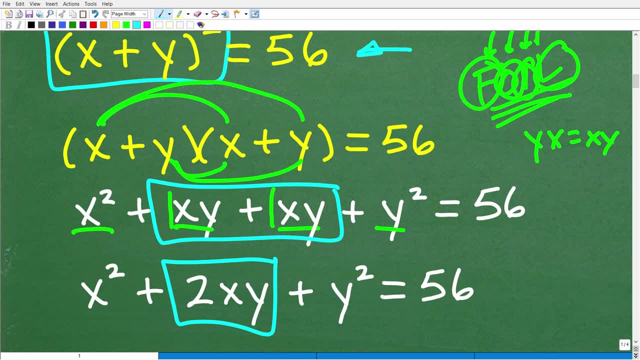 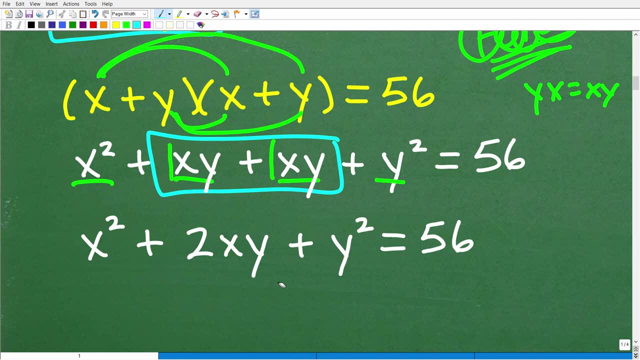 x squared plus 2xy plus y squared, is equal to 56.. Okay, so at this point in the problem, by doing this, there is a pattern that is occurring. Okay, matter of fact, there is a big, big clue going on for you to solve the problem. 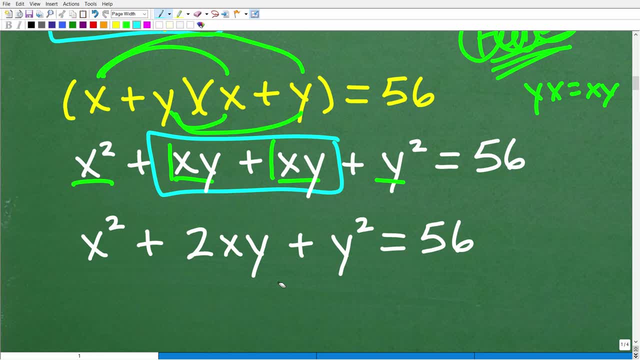 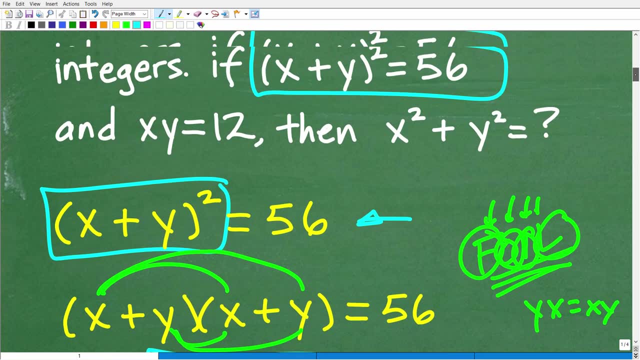 You know, as we look at it right right now, in this stage. now you might be saying, Mr YouTube math man, I'm not sure I understand what you're talking about. Well, let's go back up to the problem. Okay, just look at the information that you have And then look at the kind of status. 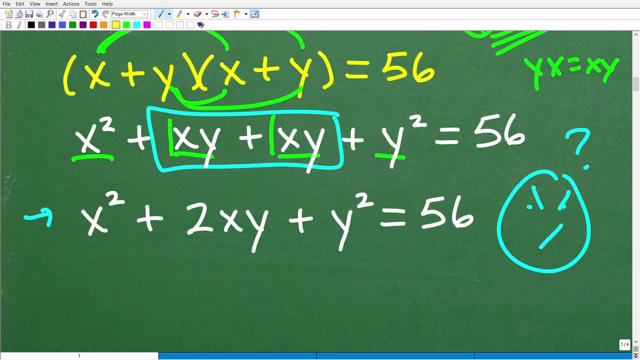 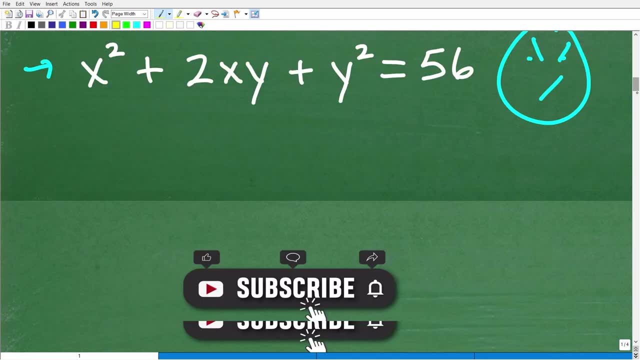 you just did. Now, if you don't understand, I will show you exactly what is the next step to solve this problem or at least to make our life much easier. So let's go to take that next step, which, of course, is having you quickly subscribe to my YouTube channel. I definitely 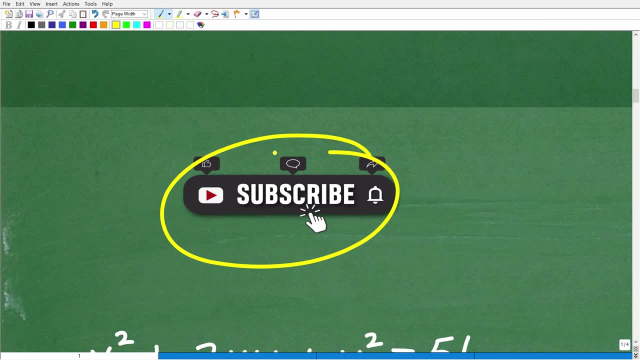 wouldn't ask you if I didn't need your support. The only way I can grow my channel, and the only reason I want to grow my channel, is to teach as much as many people math as I can. Okay, it does me no good to learn all this math. There are all these decades. 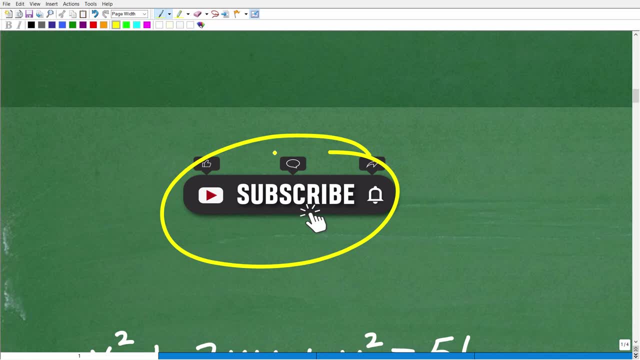 Yeah, I mean, you know I'm a teacher, right? That's what you know I'm passionate about. So the bigger my classroom, my classroom, is, the more students I have, the happier I am. So you can help me grow my reach by simply hitting that subscribe button And if you're going to do that, hit that notification bell as well. Thank you so much. Matter of fact, this is the way I look right now. 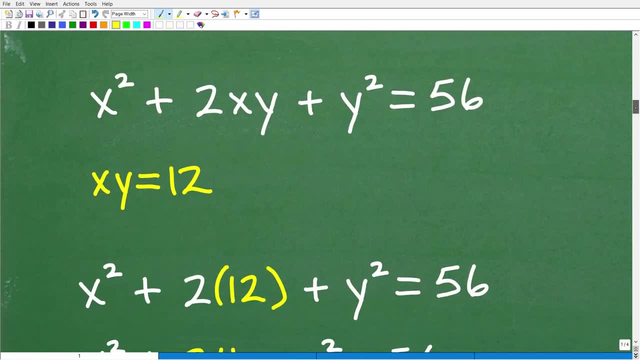 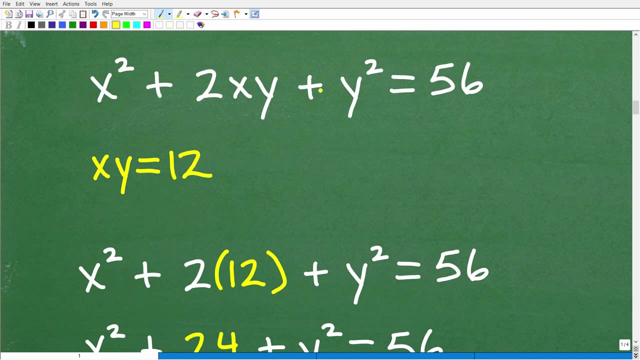 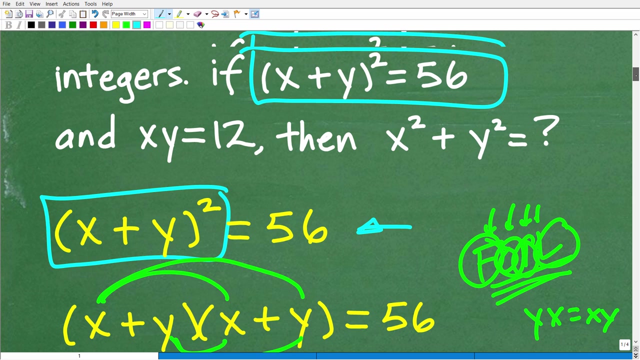 And let's go ahead and finish this problem up. So some of you might not still see the pattern here. So remember, when we had that x plus y squared, we multiply that out. then we ended up with this. But let's take a look. look at this part right here, this x- y- remember we're being told in the problem that x- y is equal to 12, right, So it kind of didn't want to tell you that explicitly because I wanted you to have a chance to figure this out on your own. 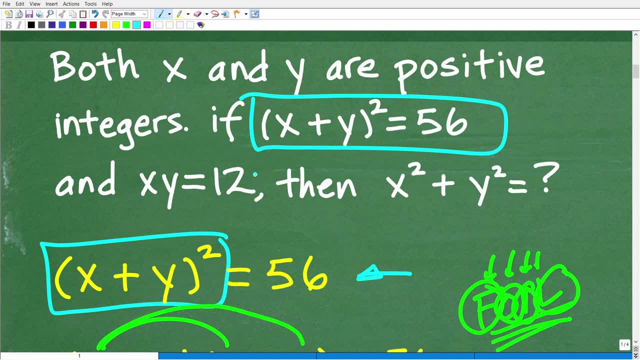 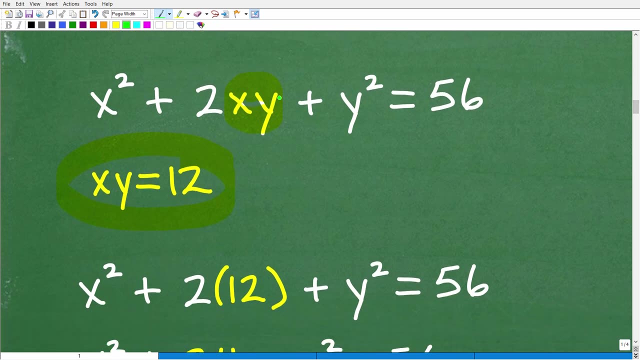 So remember, if x plus y squared is equal to 56, and x- y is equal to 12.. Okay, so this part we're going to have to use in order to figure this question out. So x- y is equal to 12.. Well, can we do anything with that? Well, indeed, we can, Because if x- y is equal to 12,- well, I have an x? y right here. I can replace this x? y with the number 12.. Okay, And when I do that, interesting things are going to happen. So let's go ahead and replace this x? y with 12.. So we'll do that. 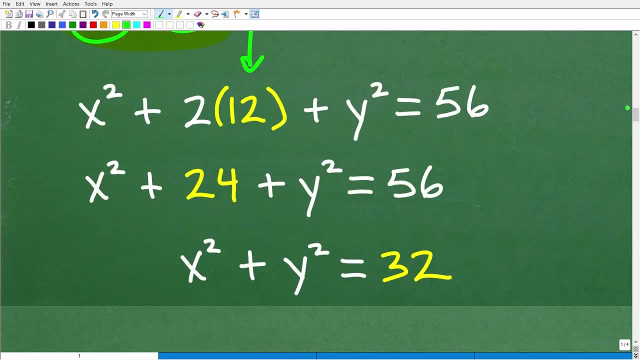 Right here And let's see what's going to occur. So that's going to be x squared plus two times, not x, y, but 12.. So two times 12 is what? 24 plus y squared is equal to 56.. Okay, so I have x squared and y squared in a 24.. So let's move this 24 over to the other side, And I could do that easily by subtracting 24 from both sides of the equation. And when I do that, what am I left on the left hand side? Well, the 24s go way. 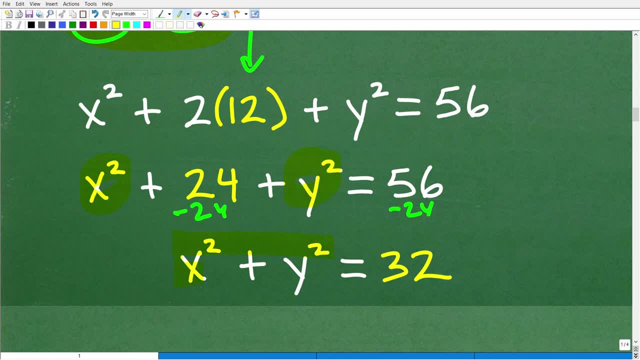 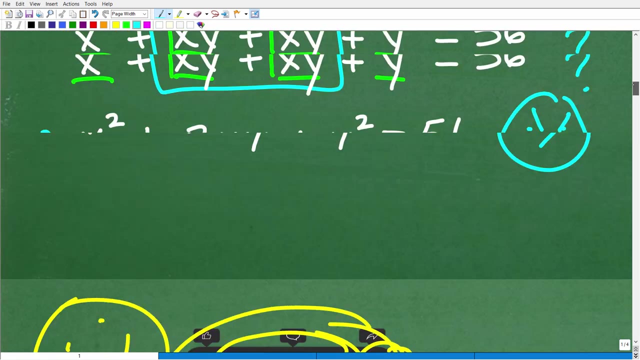 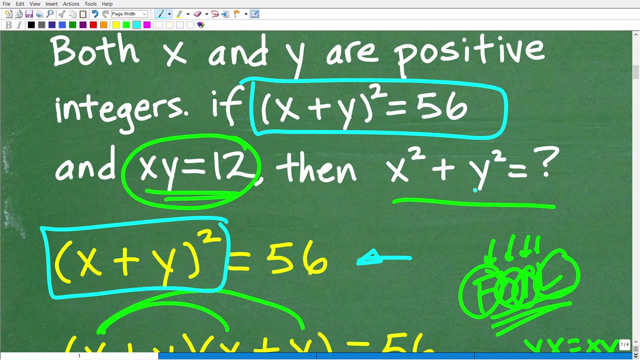 over here And I'm left with x squared plus y squared on the left hand side, and then 56 minus 24 is equal to 32.. So let's take a look at what we just have, What we just did here. we have x squared plus y squared is equal to 32.. What was the question? The question was what? Well, let's go all the way back up here. The question is: what is x squared plus y squared is equal to? if x plus y squared is equal to 56 and x times y is equal to 12?, What is x squared plus y squared is equal to? 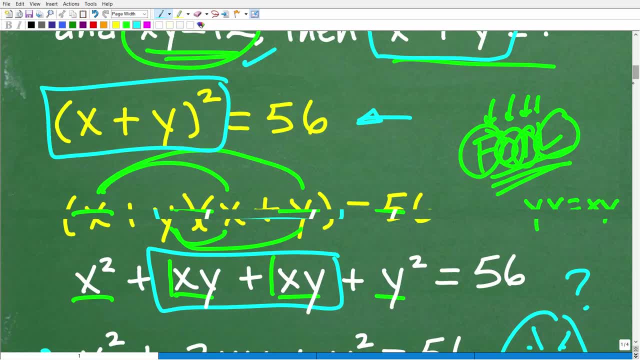 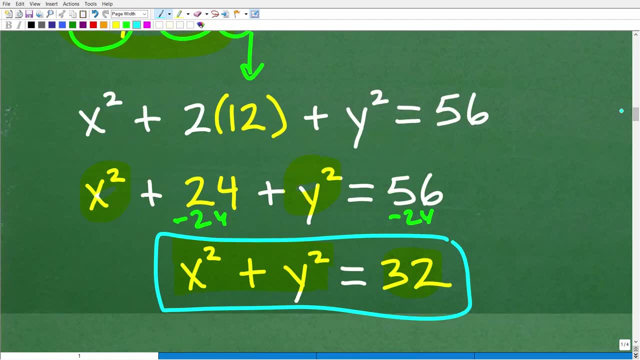 What is the value of x squared plus y squared? And of course, we figured this out without having to solve for the specific values of x and y. Okay, so here, x squared plus y squared is equal to 32.. All right, so again this type of problem or these types of prompts, and we're only looking at one here. But I guess what I'm trying to say is that problems that require a non obvious approach. okay, looking for patterns. 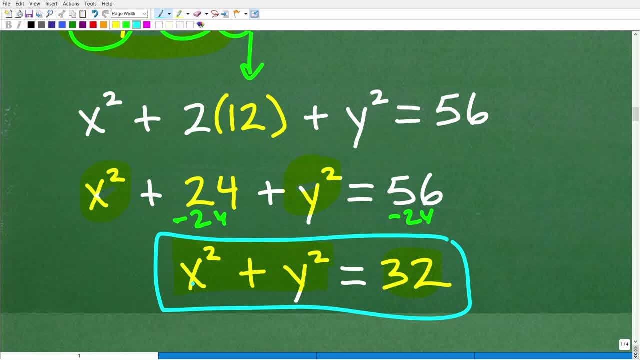 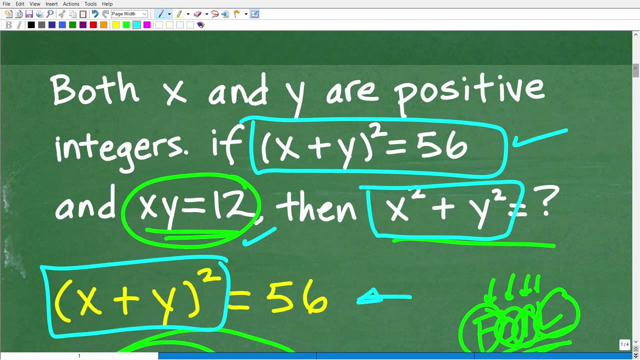 are very common type of problems on tests again, like you know, entrance exams or assessments and things like that. So be careful. when you see a problem that just seems a little bit you know kind of you know different or not so direct, It's probably implying: hey, you know, maybe start thinking about some other ways to solve this problem other than what you know is your first kind of maybe impulse right? So if you, you know, know algebra, you might be saying, Okay, well, I 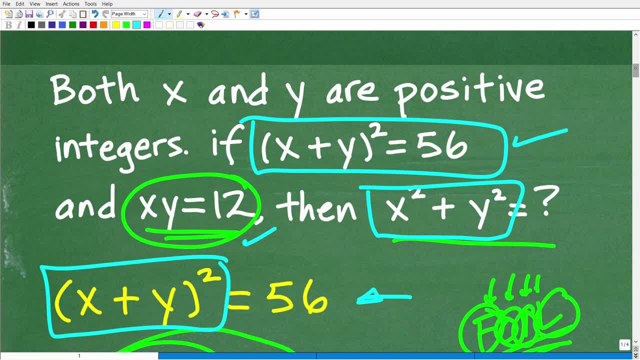 can solve for x and y here I can, you know, plug in these values And you could do that, but it's going to take you a lot more time to do that. So the only way you're going to get better at these type of problems is twofold. Okay, there's actually two, two things you need to do to improve in solving these type of problems, these kind of non traditional math problems. The first is you got to understand. you know the underlying math skills. So if you need help with algebra- algebra one, algebra two doesn't make a difference- Check out all my course links. I'm going to 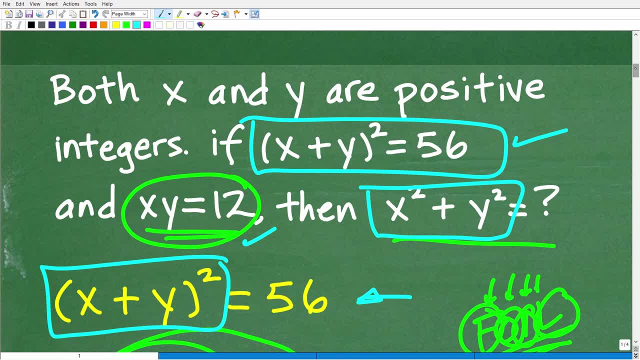 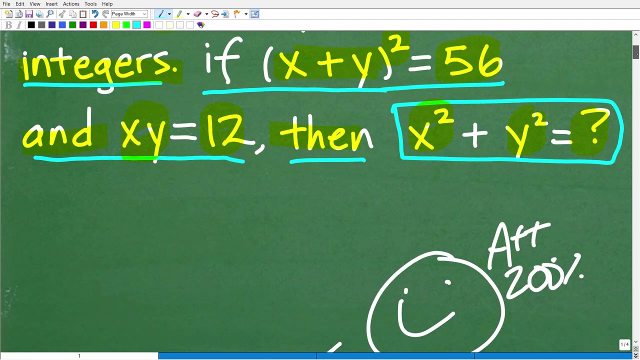 well, I'm going to leave the links to all my main courses. That's what I meant to say in the description. So they go from pre calculus algebra to pre algebra, algebra one. if you are not a math student, you want to learn math over with me, starting from basic math to algebra, geometry. check out my math skills, rebuild a course, but get your skills down first, Okay. But once you have your math skills, you know, strengthened pretty well, then what you need, what you need to do to get better at these problems, is to practice, practice, practice. Okay, that's, it's a.